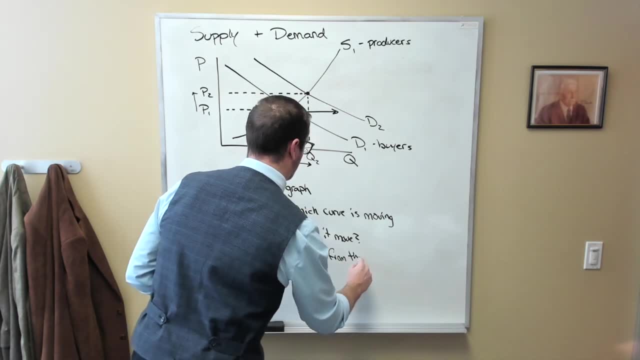 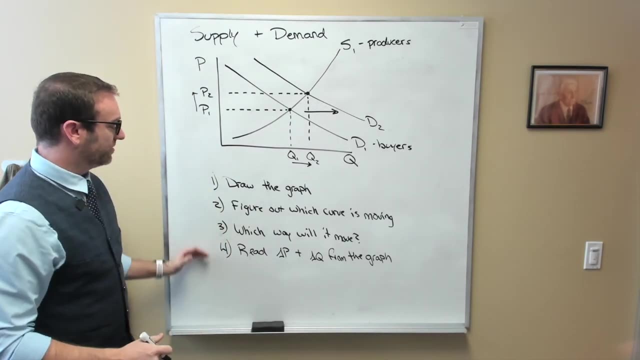 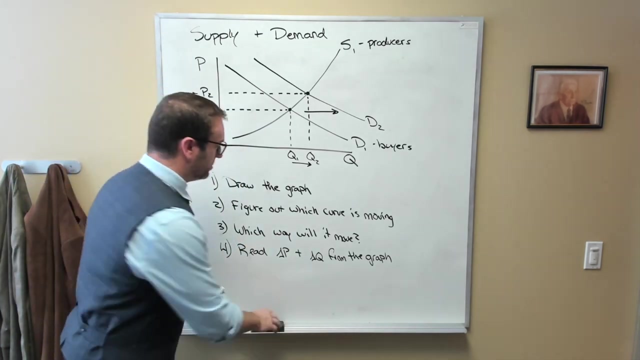 in quantity from the graph. okay, now the trick is to do these four steps in order. if you do them in order, you will get all of your questions correct, okay, so let's do a different example. so let me just kind of clear the board real fast and 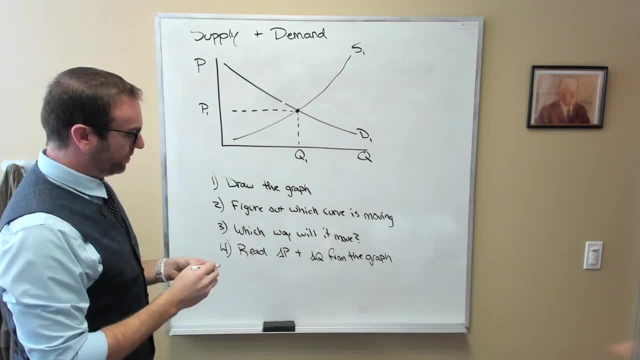 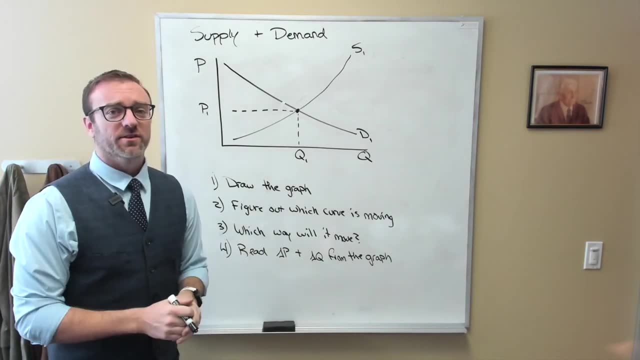 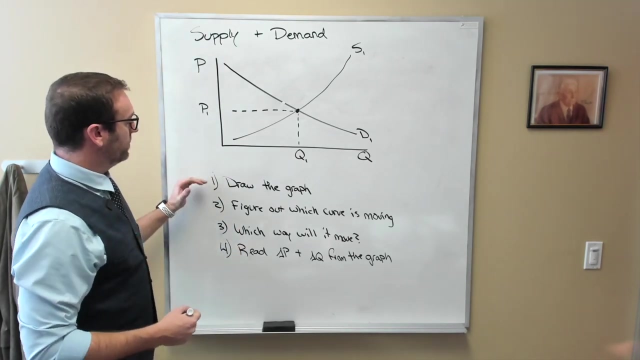 there, we are okay now. so let's pretend. instead of changing in the number of consumers, what if, instead, there was some improvement in medical care delivery or the medical care provision? well, in this case, right, we've drawn the graph. so far, there's an improvement in the technology involved. 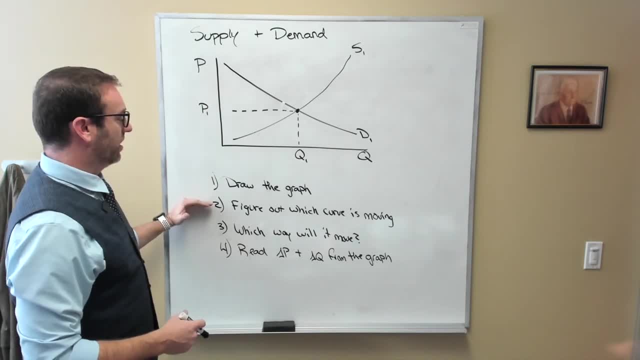 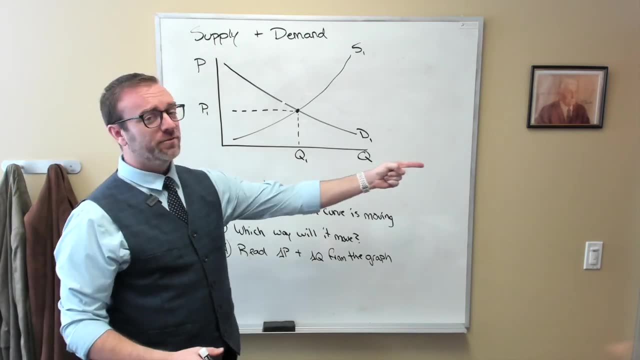 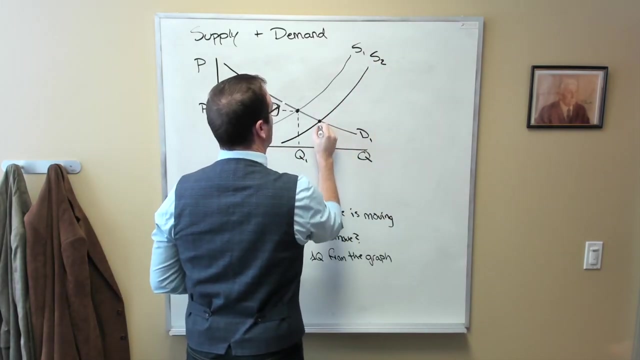 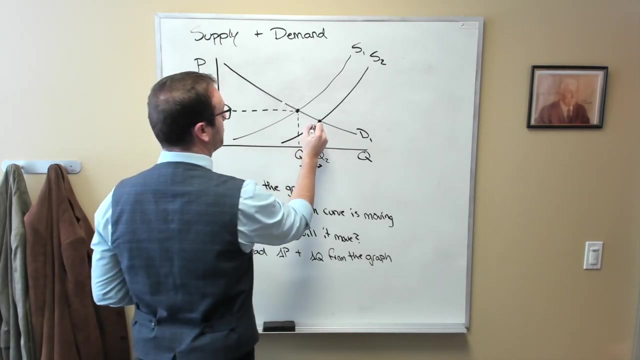 in producing health care. so that's going to affect the supply curve. you, because it's an improvement. the supply curve is going to increase, which means it's going to move to the right. okay, so let's do that. and what we can see is then step four. we can see that the change in quantity we're going to see an increase. 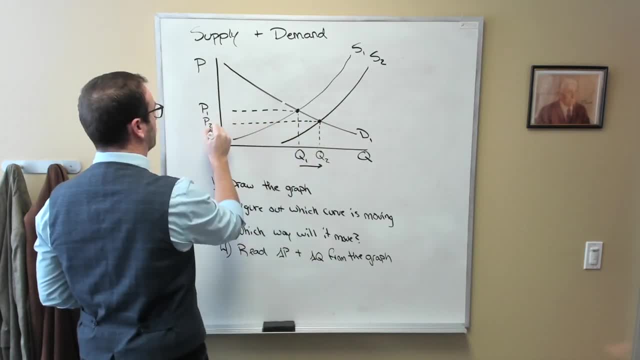 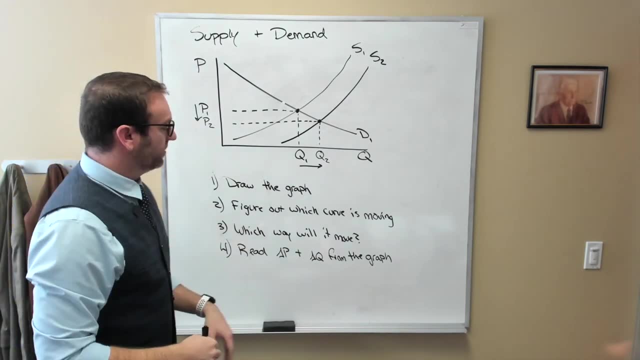 in the amount of, in this case, health care available and we're going to see a decrease in the price. okay, so this four step. okay, so this four step: we're going to see a decrease in the price. okay, so this four step, we're going to see a decrease in the price. okay, so this four step plan really does help you boil down. 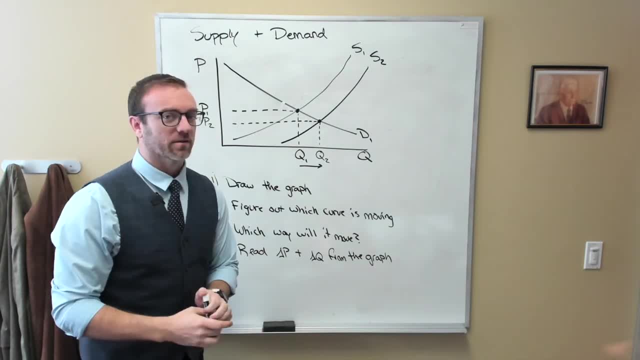 plan really does help you boil down. plan really does help you boil down what you should be doing and how you should what you should be doing and how you should what you should be doing and how you should be thinking about things. let's do be thinking about things. let's do. 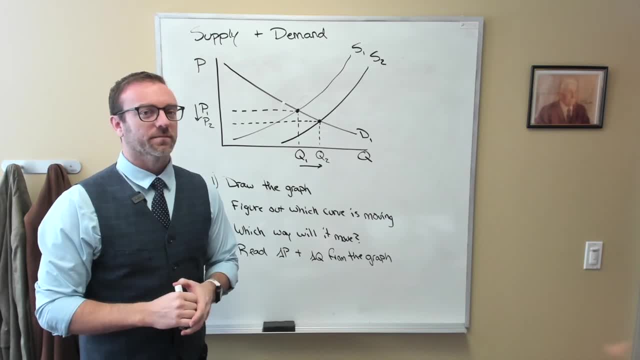 be thinking about things. let's do another example that's perhaps a little another example. that's perhaps a little another example that's perhaps a little bit more complicated. okay, so now let's bit more complicated. okay, so now let's bit more complicated. okay, so now let's do something that's going to hit, perhaps. 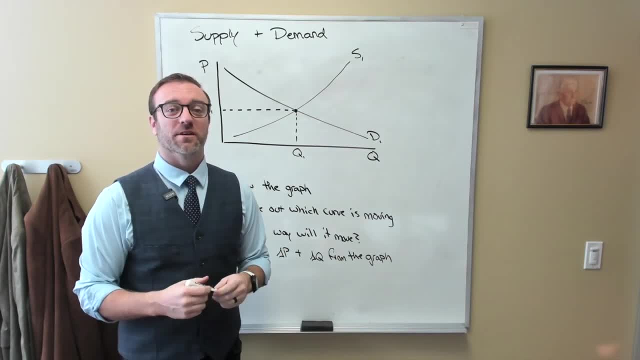 do something that's going to hit. perhaps do something that's going to hit, perhaps a little bit closer to home. let's a little bit closer to home. let's a little bit closer to home. let's pretend that we get hit with a global pandemic, because we've never heard of that before. right, And as a result of this global 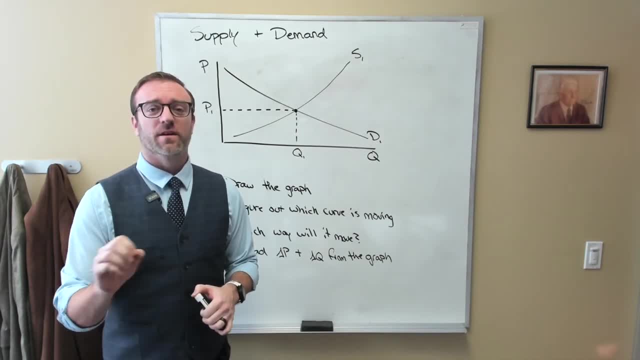 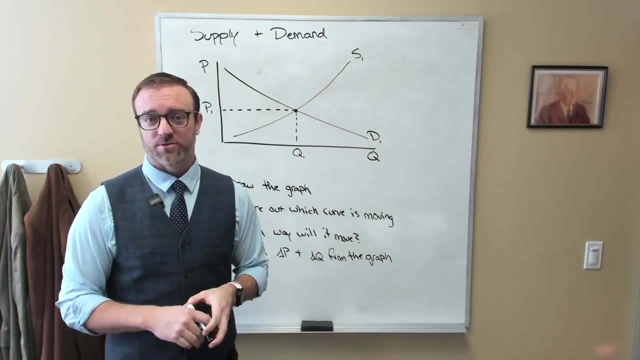 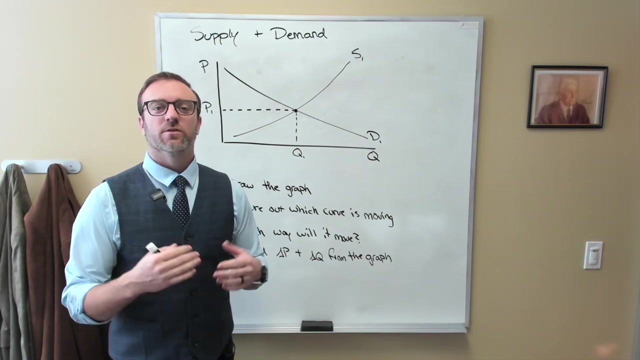 pandemic. more people are going to need healthcare than ever before. However, in order to keep the doctors and the nursing staff and all the other medical professionals safe, we impose serious restrictions on who can work, when and how frequently. So, basically, what we're going to do. 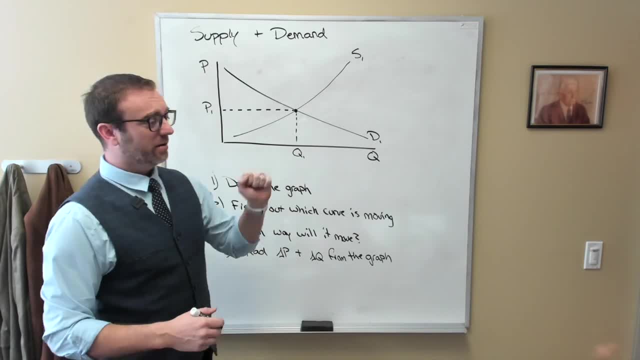 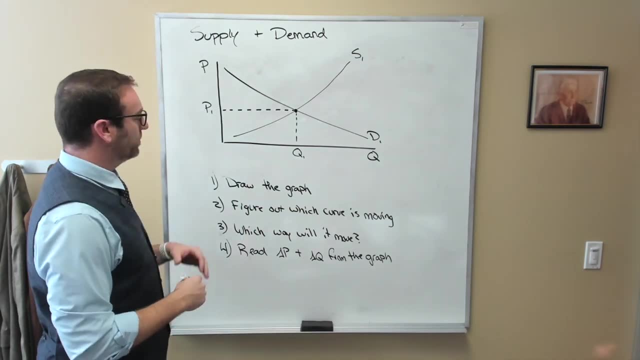 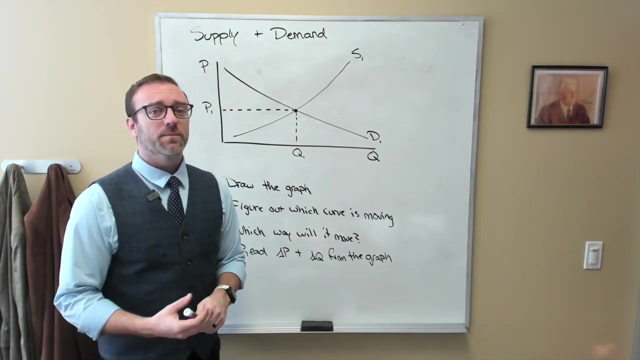 is. we're going to say that there's a higher number of people who want healthcare, but it's now more difficult to provide that healthcare. okay, So let's break this out into two different puzzles. First step: figure out which curve is moving. Well, if more people are going to want. 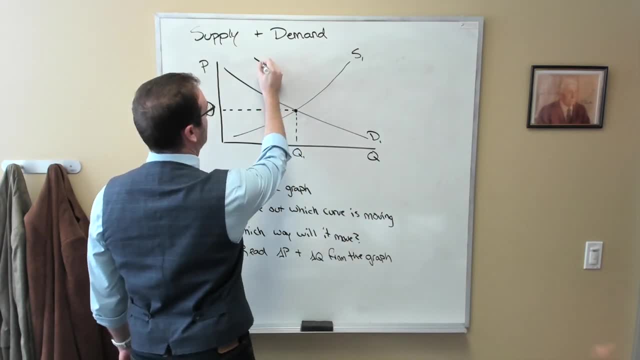 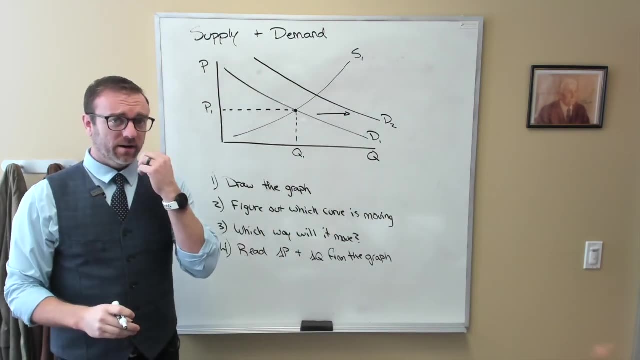 healthcare. that's an easy one. We should see an increase in the demand for healthcare. okay. So we understand that. However, if we're changing the demand for healthcare, changing the means by which healthcare is allowed to be provided, again in order to make 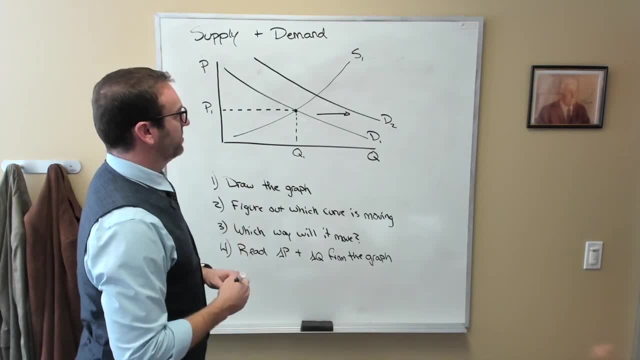 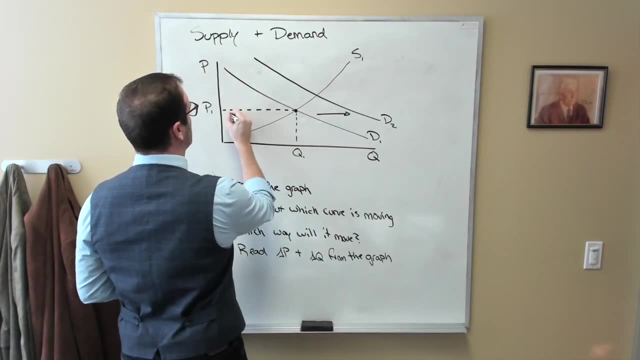 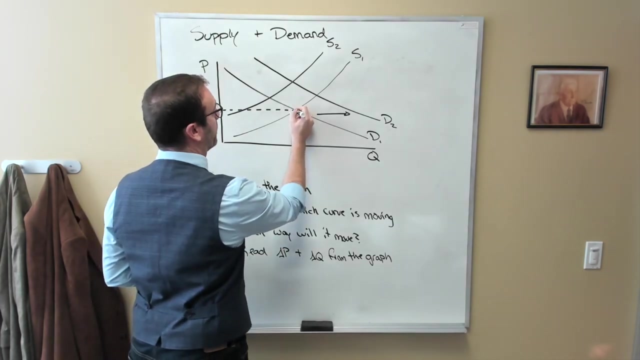 everything safer. what that's going to do is it's actually going to decrease the supply of healthcare, So we would shift the supply curve to the left. okay, So what we'd be doing is we'd be moving from our initial equilibrium point here out to this new equilibrium point here. 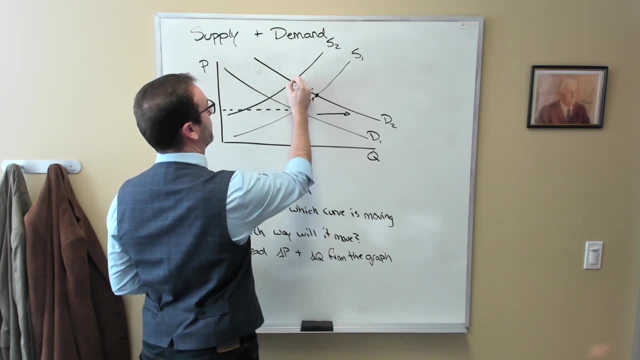 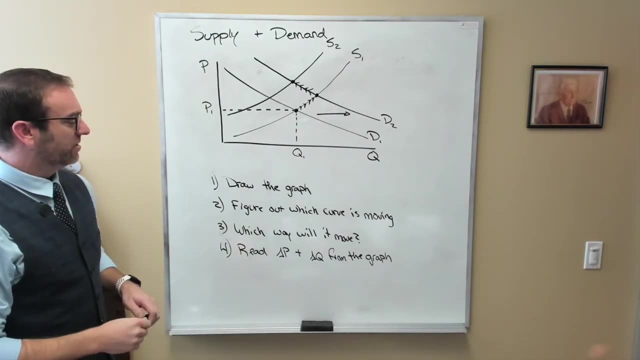 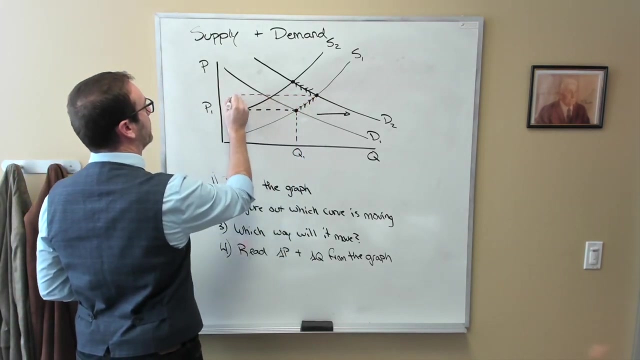 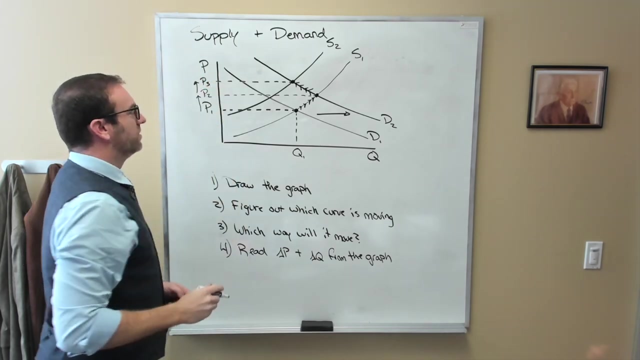 and then back up to the left, to our final equilibrium point right here. So let's think about this: How can we read changes in price and changes in quantity from the graph? Well, it should be fairly straightforward that price is going to go up, So we understand that. But what about changes? 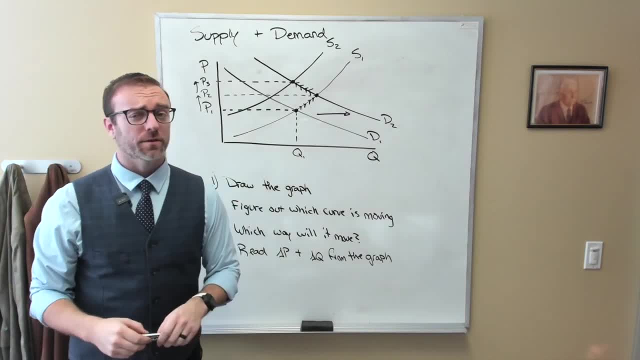 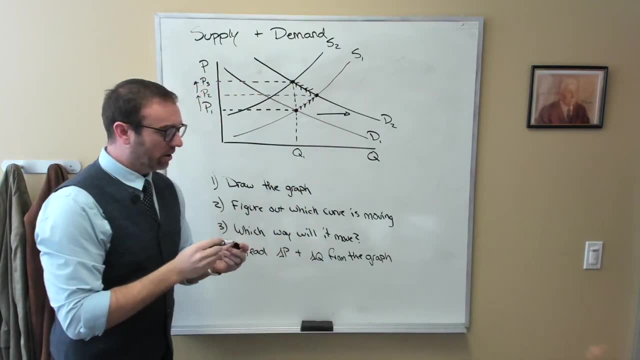 in quantity Now. I have deleted a lot of my data. I have deleted a lot of my data. I have deleted a lot of my data. I have deliberately drawn this example to show you that in this case, there is effectively no change in quantity whatsoever. However, we should be very careful in concluding. 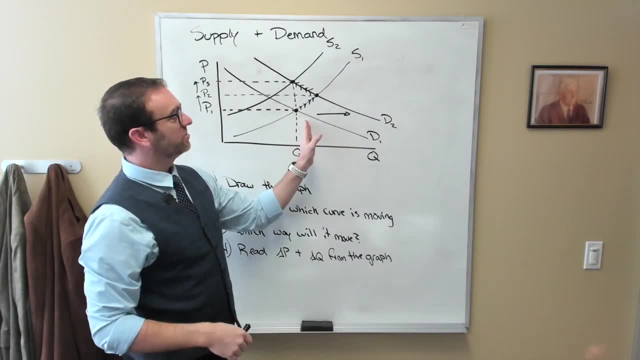 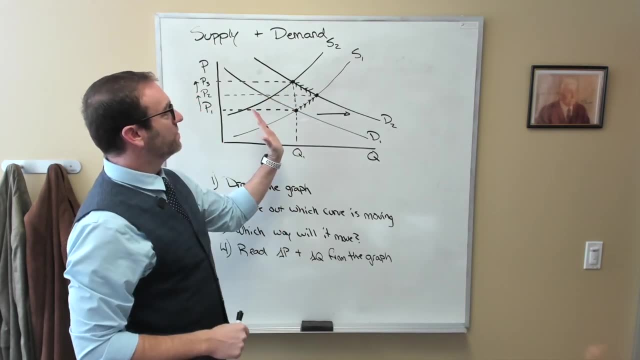 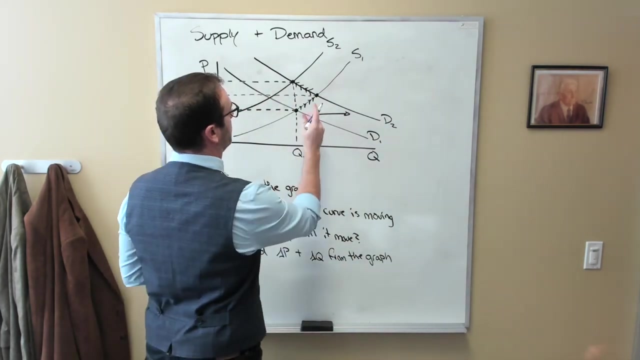 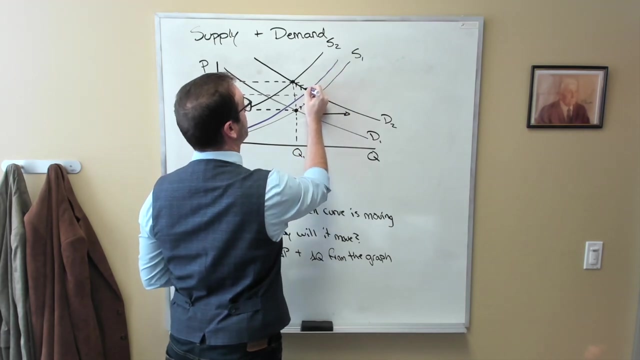 that there is no change because it depends on how much the demand curve shifts out to the right compared to how much the supply curve shifts to the left If the demand curve shifts further to the right than the supply curve. so, for example, if we had a big increase in demand here and only a very small increase in supply or decrease in. 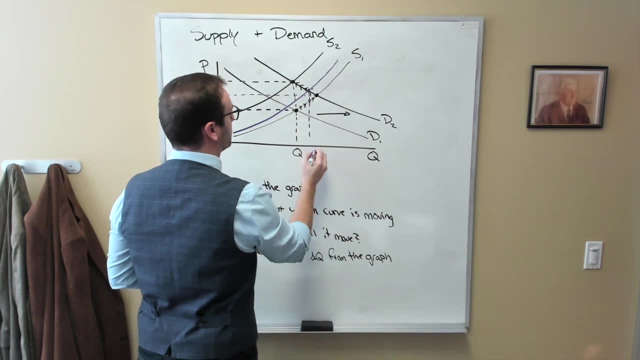 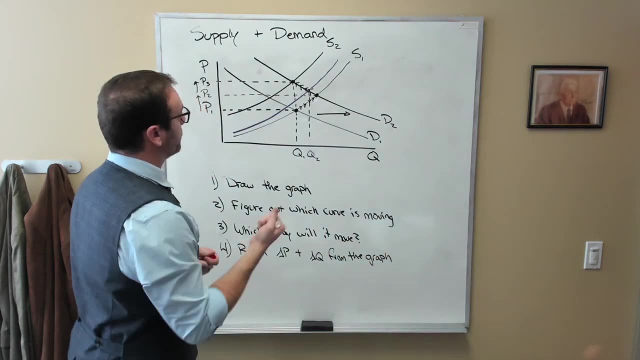 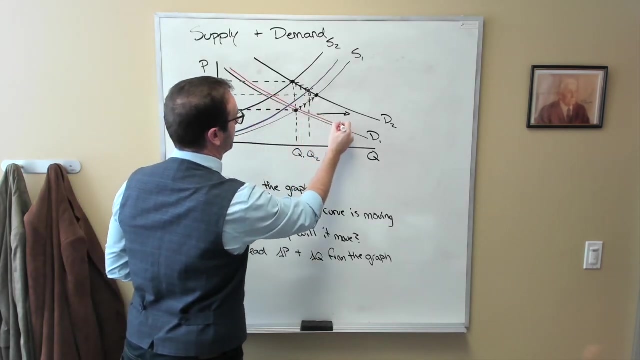 supply, well then we would get an increase in price but an increase in quantity. Conversely, if we had a very small increase in demand but a very large decrease in supply, well then that would be something like this, And we would see our equilibrium point being here: